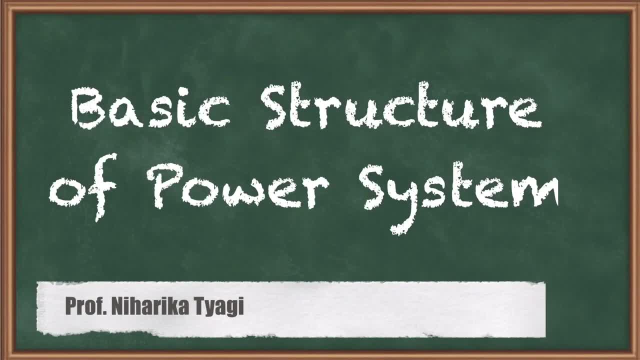 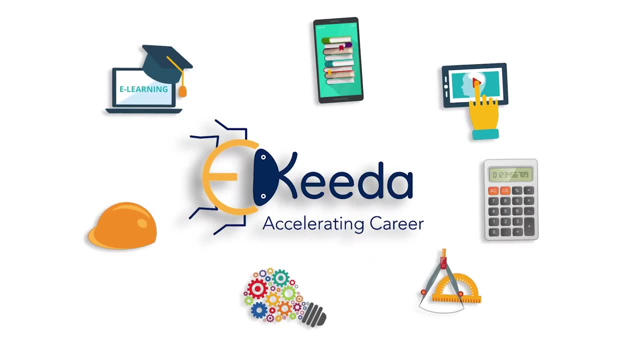 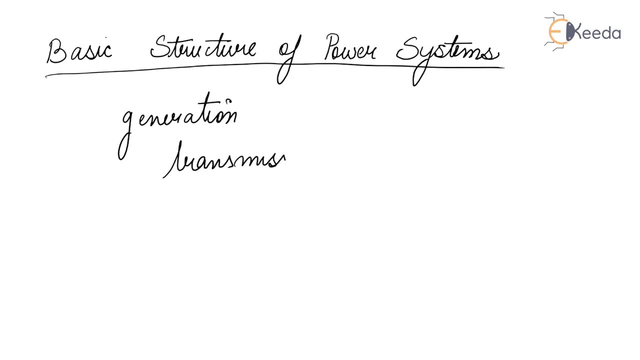 Hello friends, welcome to eKIDA. Title of the lecture is Basic Structures of Power System. What is power system? Basically, it is a network which deals with generation, transmission, distribution and utilization of electrical power and electrical devices connected to system, including generators, motors and transformers. Basically, electrical power systems are comprised: 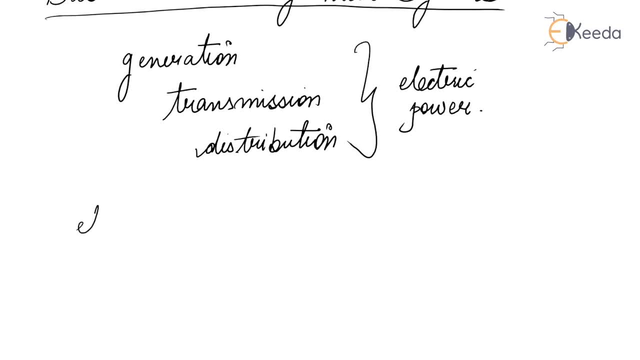 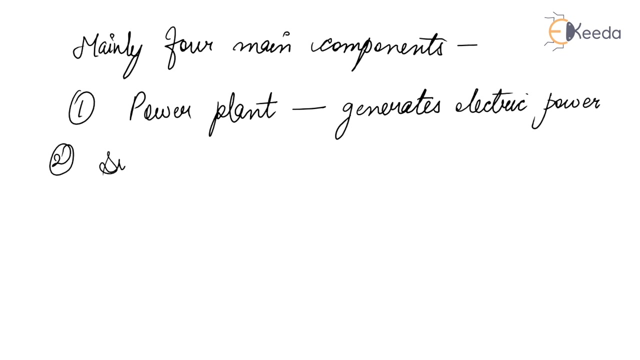 of components that are connected to produce electrical energy and transmit this energy to consumers. So mainly 4 main components are there. First is power plant, which generates electrical power. Second is substation. We have voltages, step up or step down, to carry. 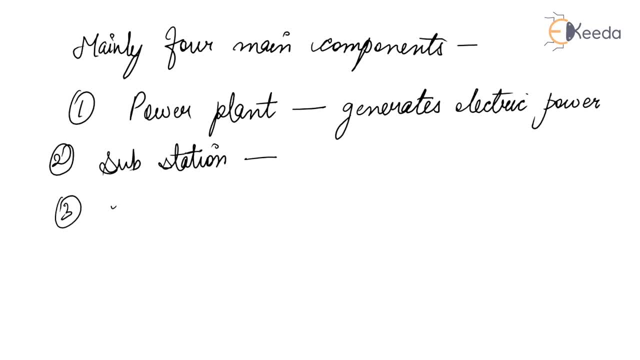 power over long distances. This is a power plant that generates electrical power over long distances. andury and electricity is being collected over long distances. This power plant lines or cables. Then third is transmission lines. It is used to carry bulk amount of power over long distance. And the last one is distribution lines, As name itself say. 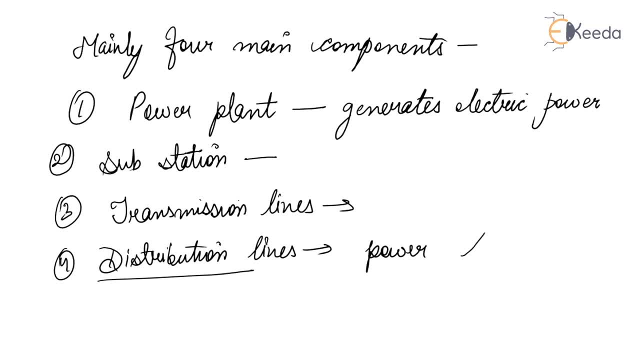 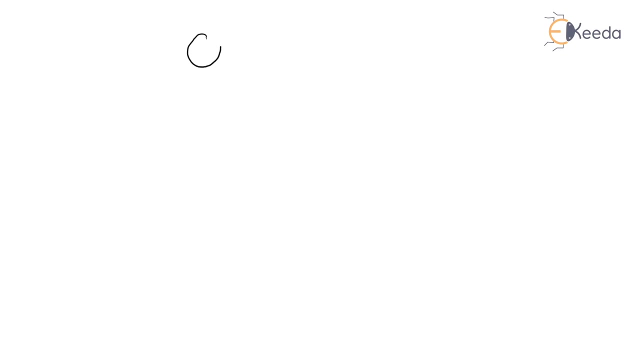 it is used to distribute power to the consumers at lower voltage level. So main four components are there: power plant, substation, transmission line and distribution line. Now layout of power system. First, power is generated at the middle station at a voltage level of 11. 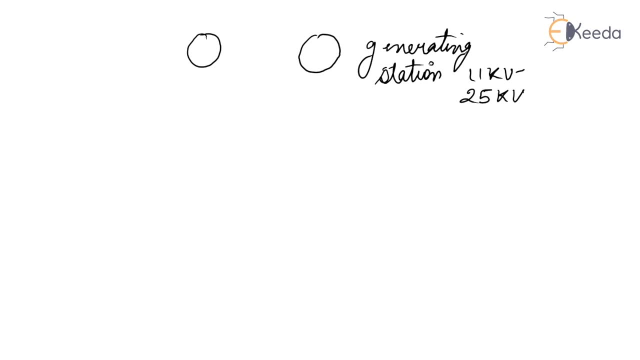 kV or at most up to 25 kV. Then this voltage is stepped up at transmission level, So this will go from 220 kV to 400 kV. See. transmission of electrical power at high voltages has several advantages, including the saving of conductor material and high transmission efficiency. 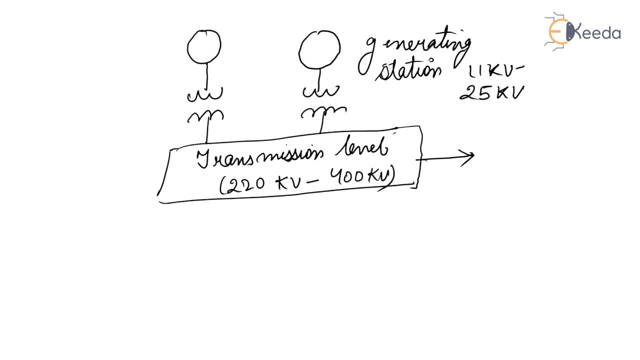 Here electrical power is transmitted to the outskirts of the city. So from the fact we know Guwahati, utilization as per the energy consumption is low than compared with metropolitan cities. So to tackle with this difference between power generation and power utilization, this power is transmitted to the metropolitan cities. through tie lines to other systems. Then voltage is reduced by step-down transformer to 33 kV at sub-transformation. One generator is also there to feed extra power into the network. Then again, this voltage is stepped down using step-down transformer. at distribution level: primary distribution. 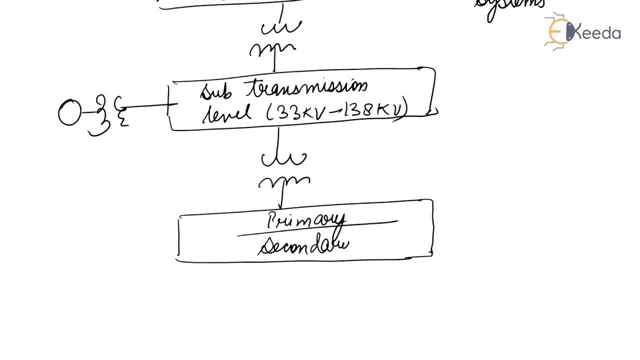 to medium-large consumers at 11 kV and secondary distribution to small consumers at 440 V to 30 V: 440 for three-phase, 230 for single-phase for industries and domestic application. Then it is adapted to belong to other devices. The power generation is also done based on. 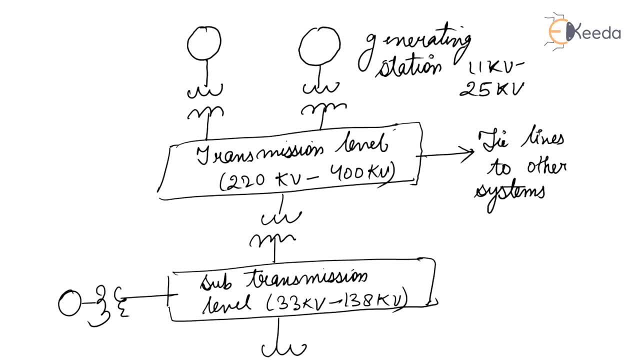 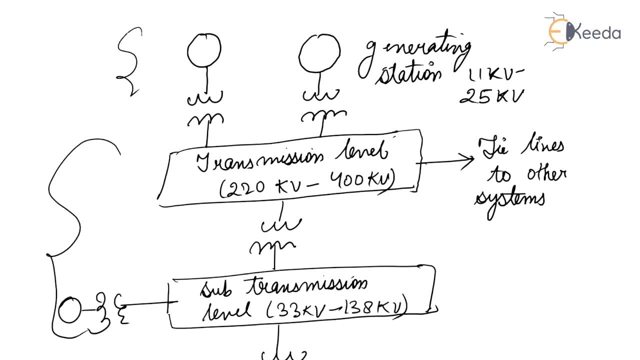 this definition. So it is not controlled by the power supply system Here, this voltage. As I told you, basically it is a network which consists of generation, transmission and distribution. So the question is: why not generate 400 kV, no need of transmission? 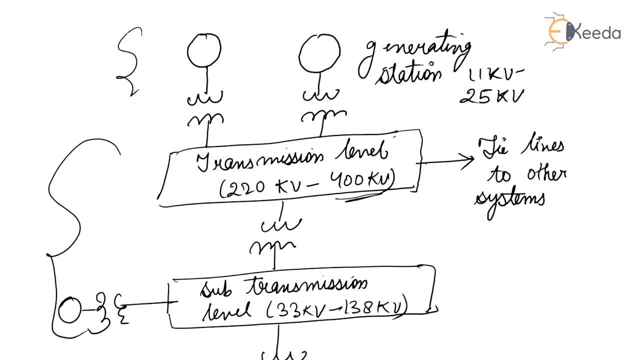 Then the reason is because of problem of cooling, insulation material. we can go at most up to 25 kV Higher the voltage, lower will be the current. In fact, bulk transmission is possible only when the voltage is high. You all know power transmission is directly proportional to the square of the voltage. 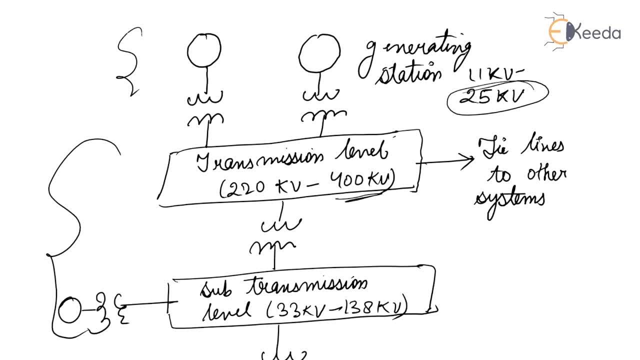 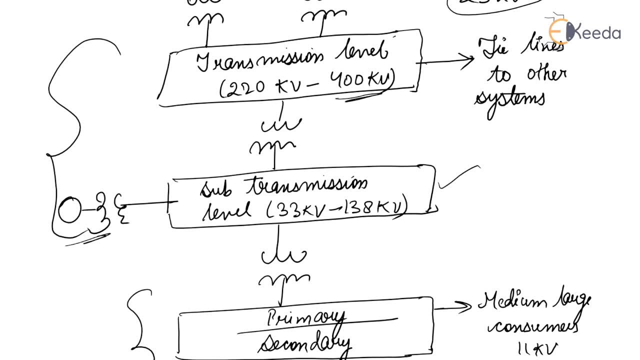 Higher the voltage, more power you will be able to transmit. Then there is a sub-transmission level. There are large consumers, so you can have a generator also to fed extra power into the network. Then again, transformer, step down transformer. we have reached a distribution level. 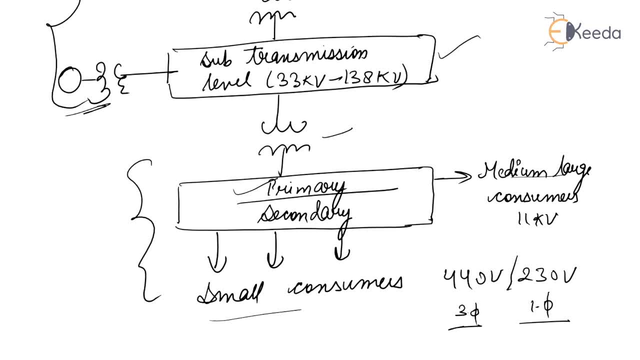 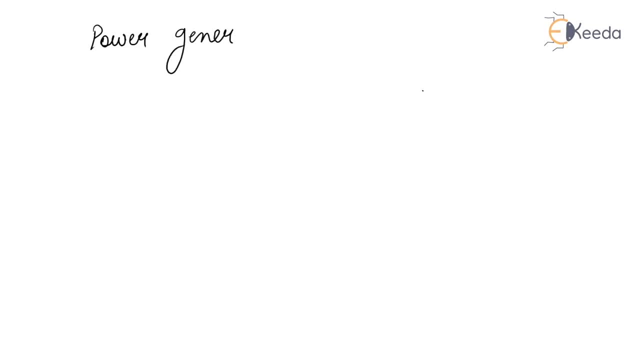 Primary distribution to medium, large consumers. secondary distribution to small consumers. So network consists of power generation. Multiple possibility of power generation is also possible here, And so this is what is called power generation. power generation range is 11 kV When you compare power generation and power plant to charge current power.